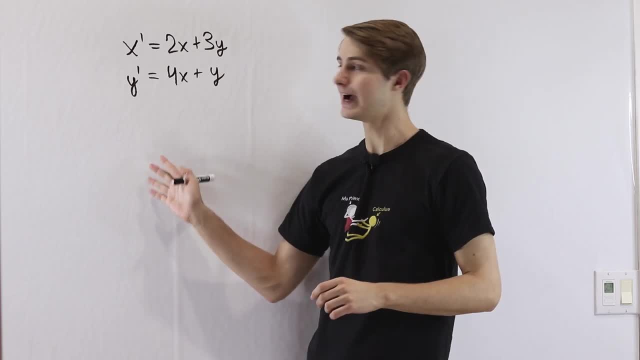 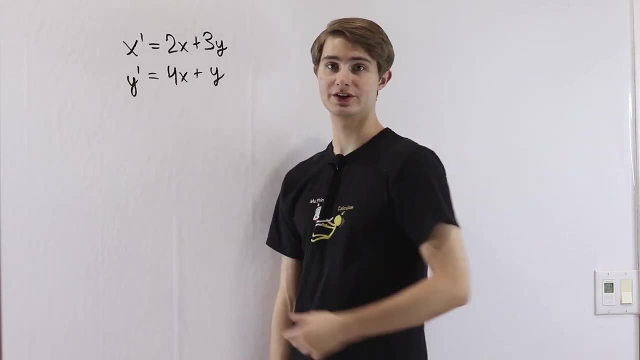 as water circulates between them. But we're just going to consider in the abstract how do we deal with this kind of equation? Now, the first thing to notice is, obviously, this is a system of differential equations, So we have two different dependent variables. x and y are both going to. 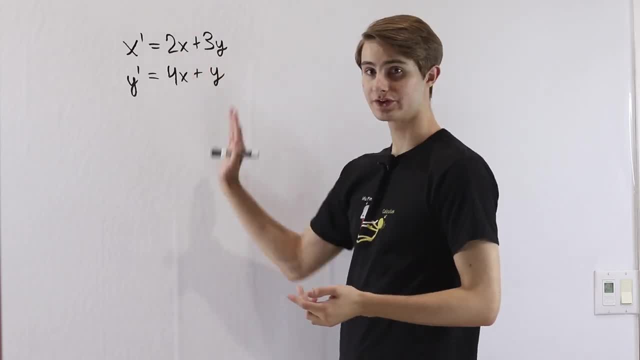 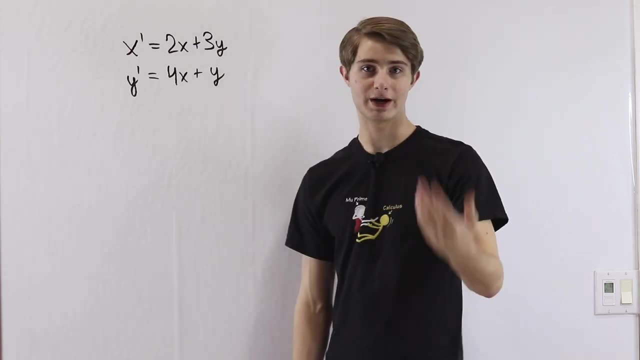 depend on something else like t, and we want to solve for x and y in terms of t. In order to do that, we want to start looking at this equation and thinking about what it reminds us of. What does this sort of look like? That might be something that we want to solve for x and y in terms of t. 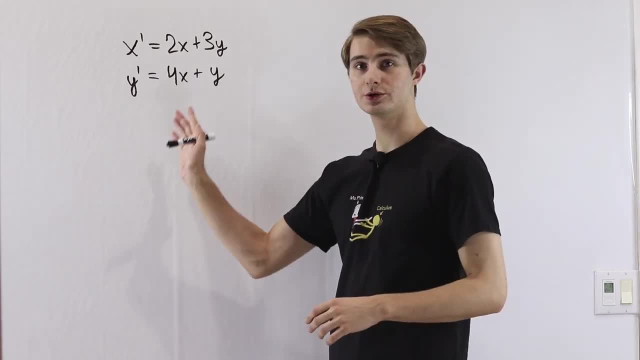 What does this sort of look like? That might be something that we want to solve for x and y in terms of t might allow us to simplify the equation down, because dealing with two equations at the same time is kind of hard, So we maybe want to try to compress it into one equation In order to do that. 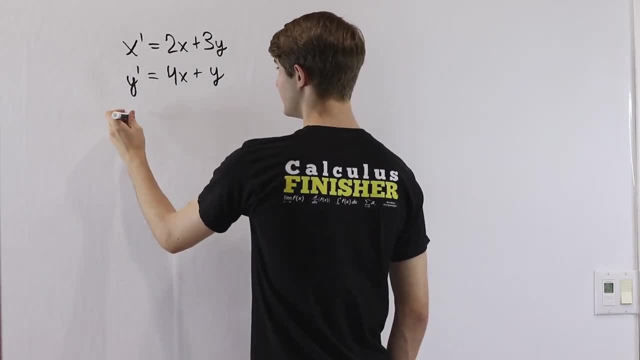 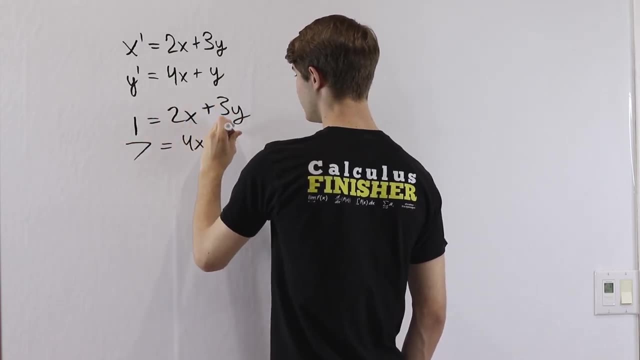 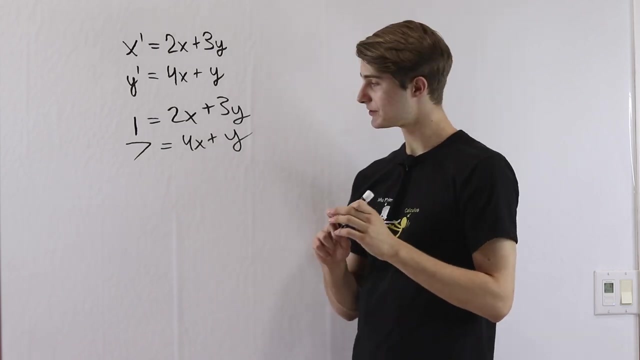 I'm going to present a different type of equation. If we had 1 equals 2x plus 3y and 7 equals 4x plus y, This is a system of equations. It's not differential equations anymore. This is just solving for x and y as numbers, One way that we can solve this kind of. 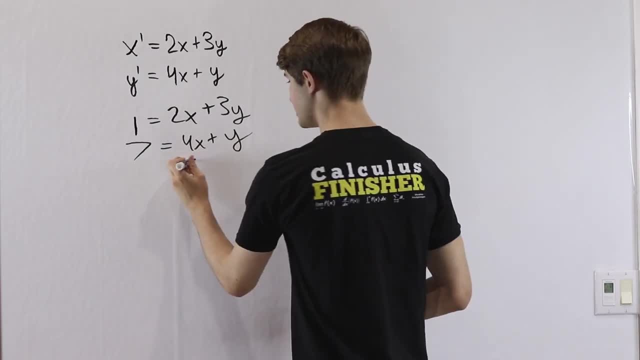 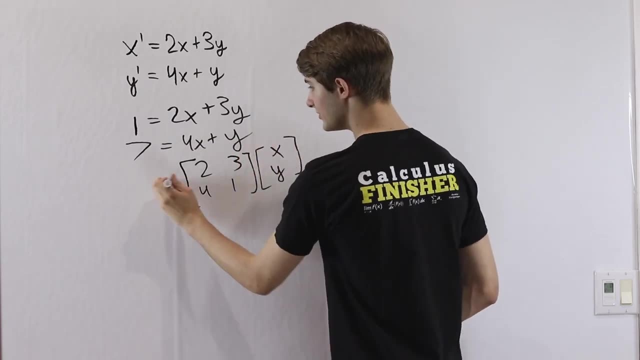 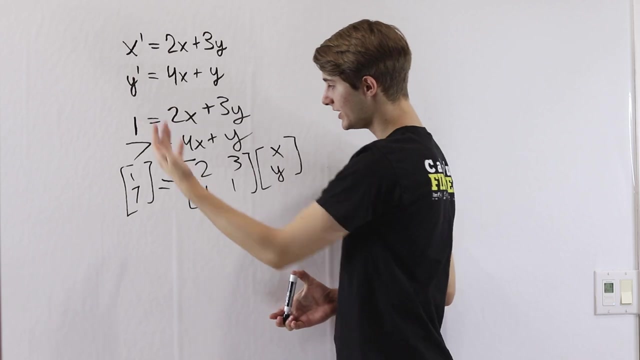 system is to write the right side of the equation as the matrix: 2, 3, 4, 1 times the vector x, y, and set that equal to 1, 7. And this is helpful for us because it takes two equations and turns them into one equation, which lets us do some fun manipulations that are otherwise pretty difficult. 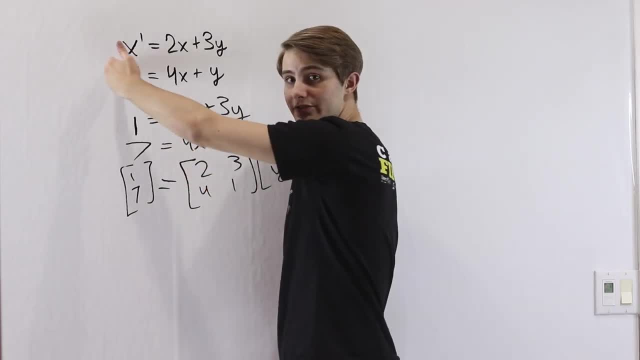 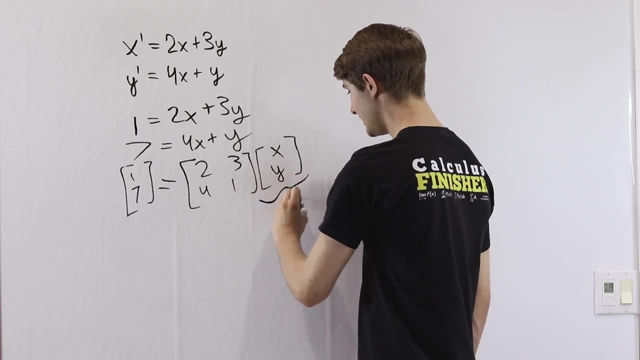 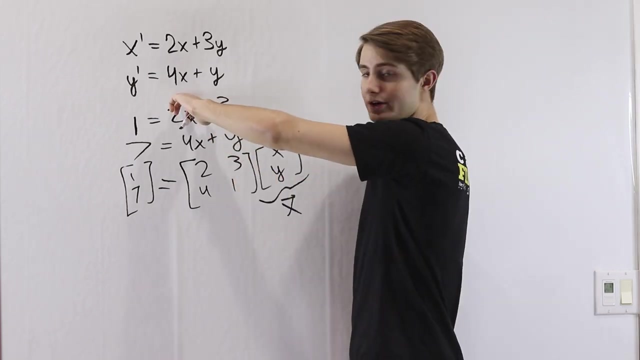 So maybe we want to take this idea and apply it to the differential equation that we have here. In order to do that, I'm going to call this x y, vector x, with an arrow on top of it to show it's a vector. This is going to denote the vector x- y. So when we look at our equation up here, we're going: 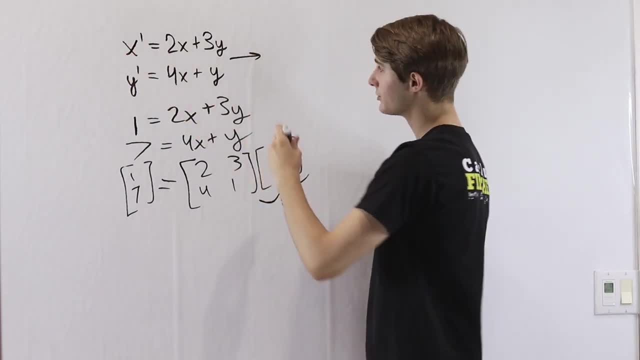 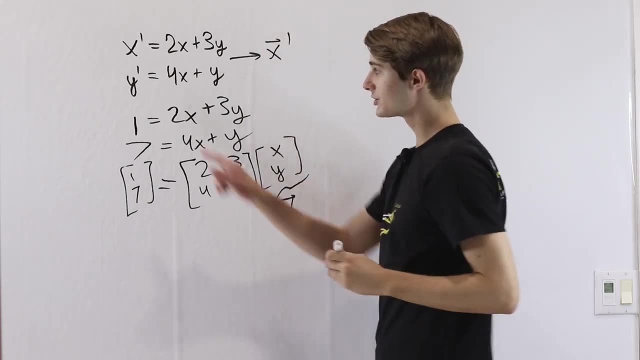 to rewrite it. and when we look at the left side of the equation, Notice x, prime, y. prime is the derivative of x- y, So we can actually write the left side as x vector and then prime That's going to equal over here as 4x. 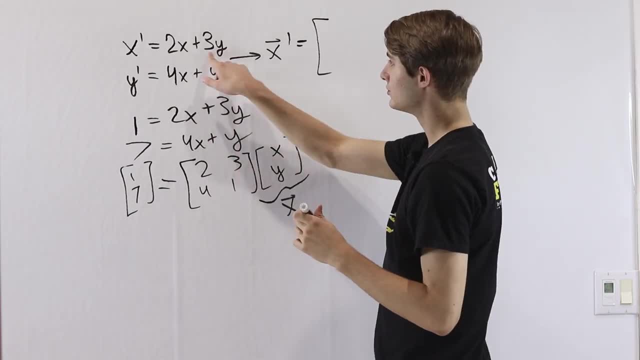 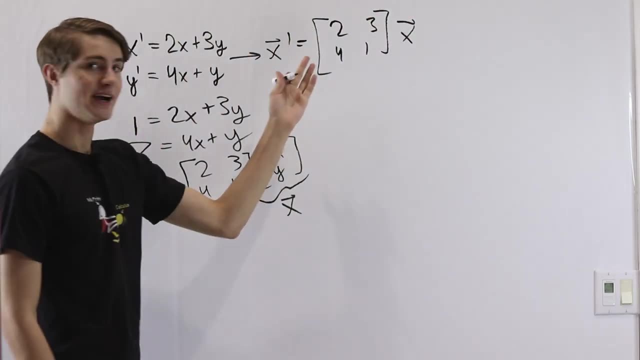 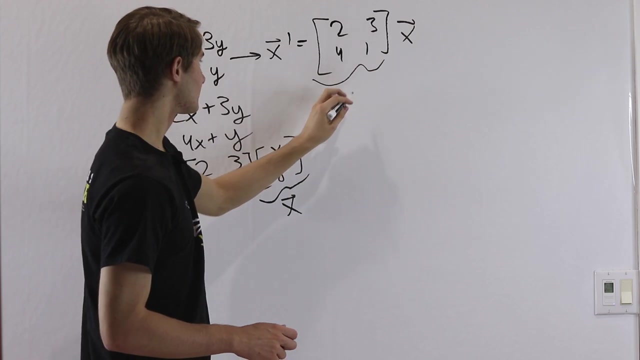 we do the same matrix multiplication that we did here. So this two, three, four one becomes two, three, four one, and we multiply that by the vector x. So this is our new differential equation. I'm going to call this matrix A just to make things a little easier for us. 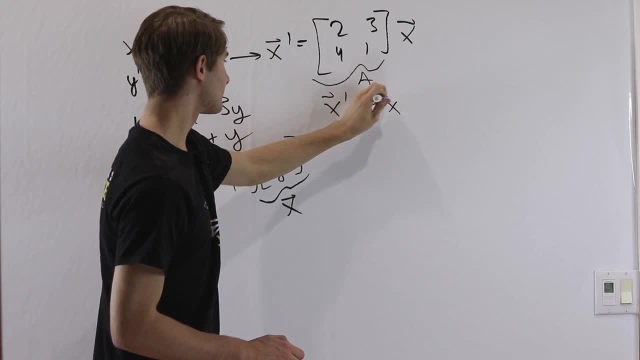 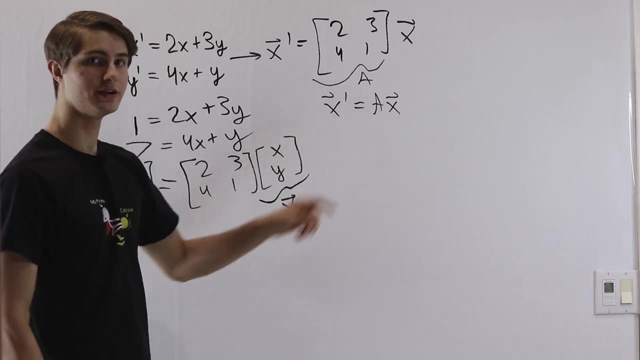 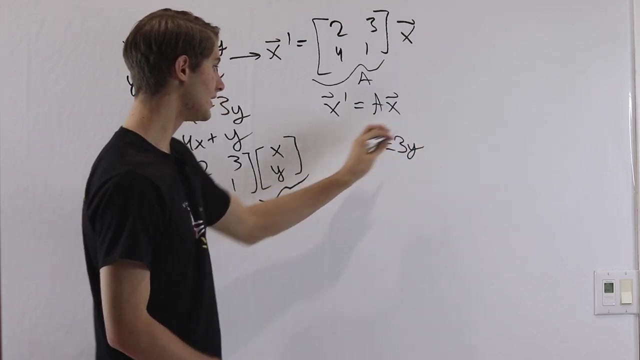 So we have x vector, prime equals A, x, And one of the things that we might notice at this point is that this differential equation here kind of reminds us of something else, which is, if we think about, for example, y, prime equals three y. If we wanted to solve 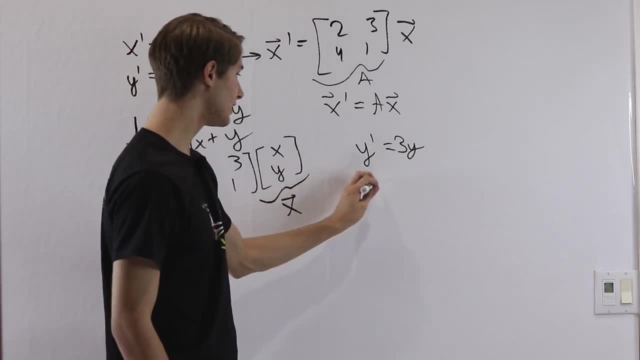 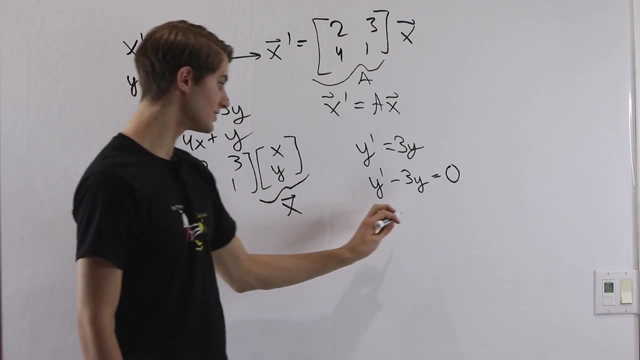 a differential equation like this, what we can do is subtract three y on both sides, So we have y prime minus three. y equals zero, And then this is a homogeneous differential equation. So we would guess y equals some constant c times e to the r t, And this is 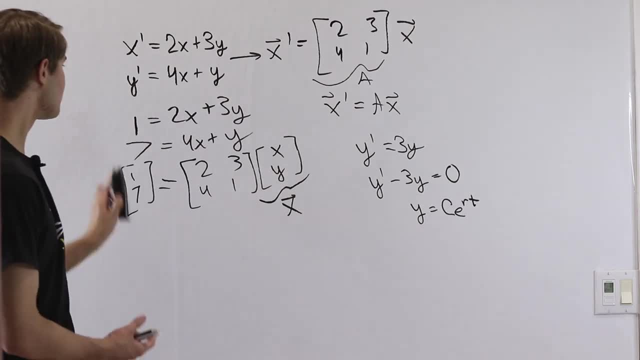 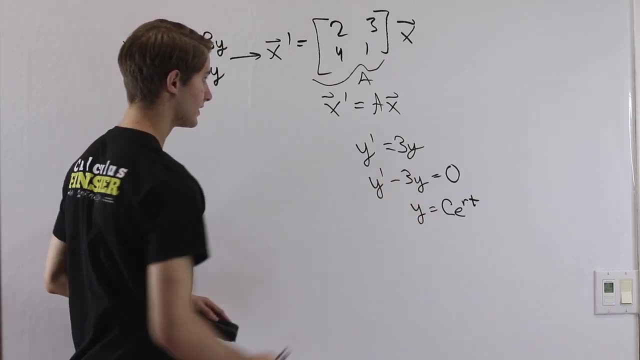 what we're going to do. We're going to take this value and we're going to multiply it by two, three, four, one, and then we can go through the equation to try to find the correct value of r. So when we look at the equation that we have here, maybe we want. 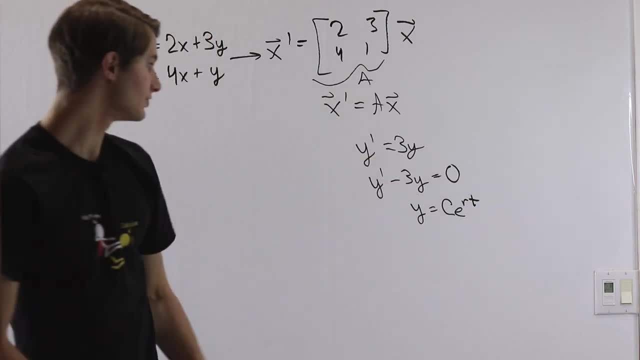 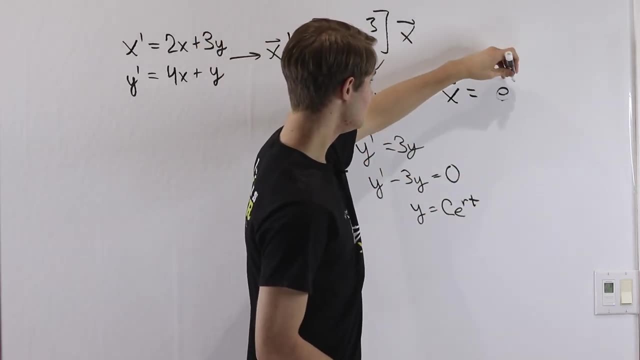 to think about applying this same kind of idea. So we want to think about what we're going to set x equal to. for our guess, We want x to be equal to. well, we know it's going to be something times e to the r, t, But remember that x is a vector, So e to the. 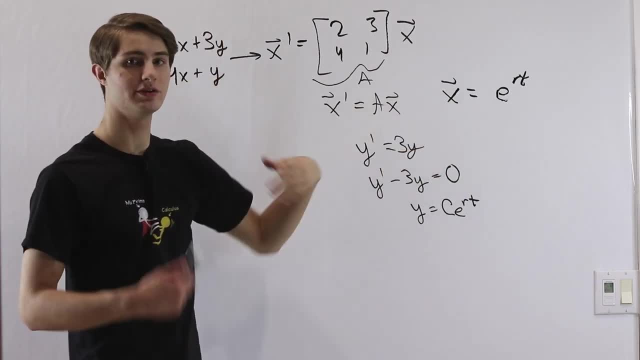 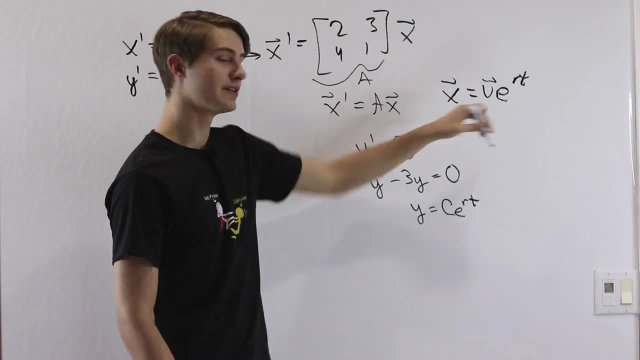 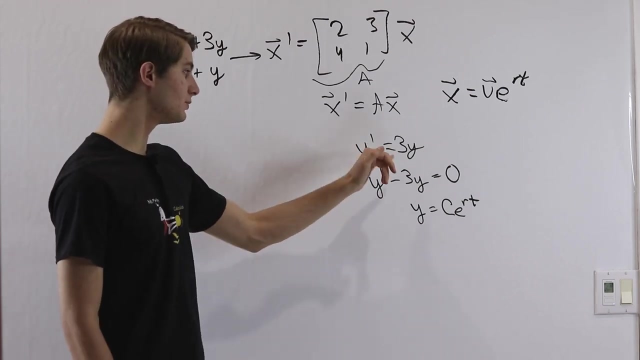 need to multiply this by some vector in order to turn it into the vector that we want. So, instead of having a constant c, we're going to have some vector of constants that I'll call v. So this is our guess for what x is equal to, because, just like with y, prime equals. 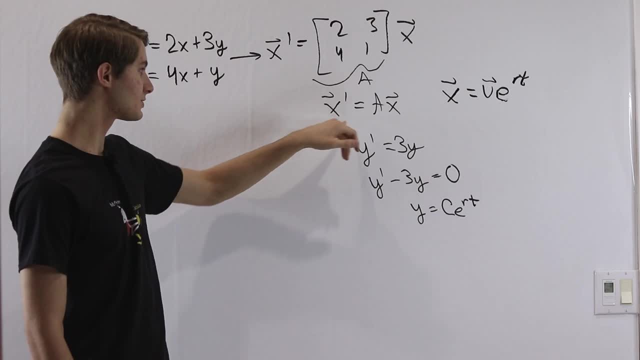 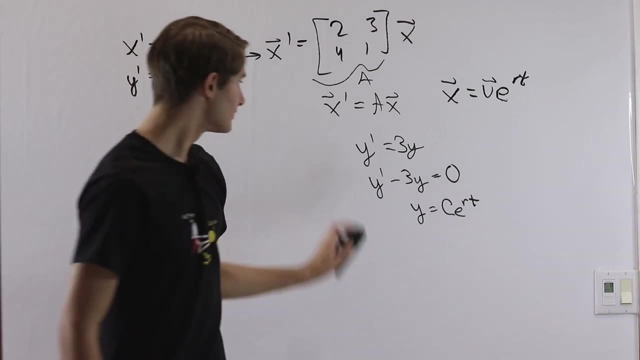 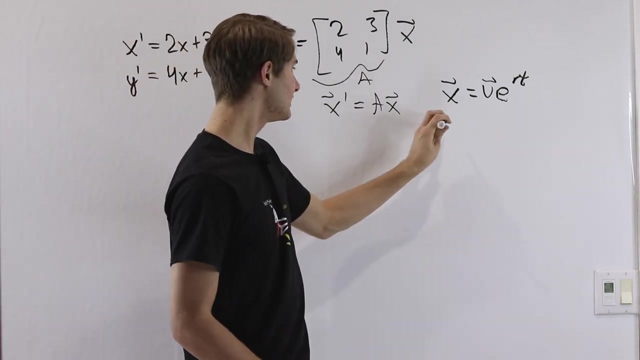 3y, doing the derivative multiplies it by 3, when we have x prime equals, ax, doing the derivative multiplies it by this matrix. So let's give ourselves some space and try to go through this problem here. When we differentiate x, we're going to get x prime equal, to remember. 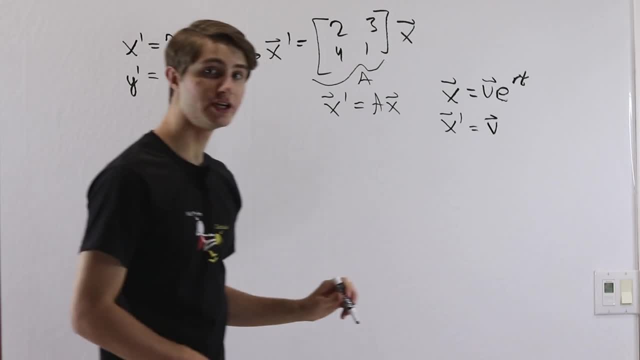 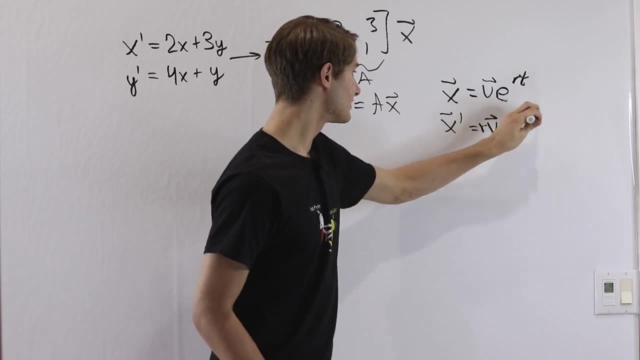 v again is a vector of constants. so that's not going to change at all when we do this differentiation. But when we have e to the rt differentiating, that gives us r times e to the rt. So now when we go back to this equation, we're going to have a vector of constants and we're 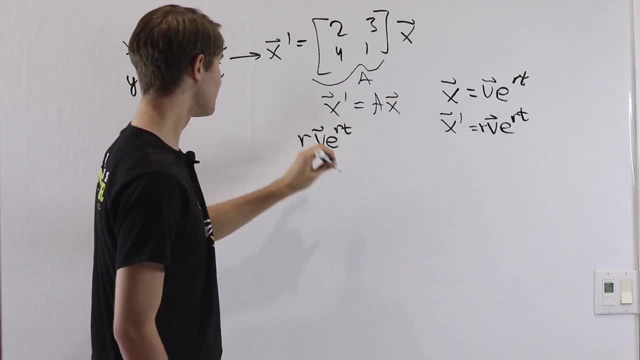 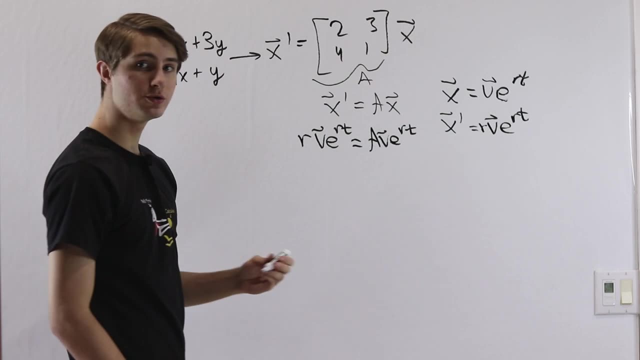 going to have r v e to the rt on this left side. equal to a times x is v? e to the rt. And again, the cool thing about this, we have e to the rt, e to the rt, so those are going. 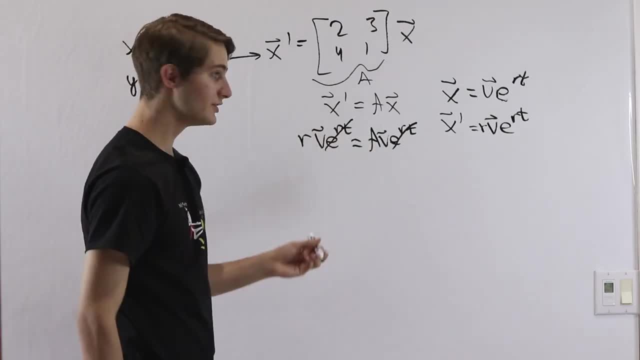 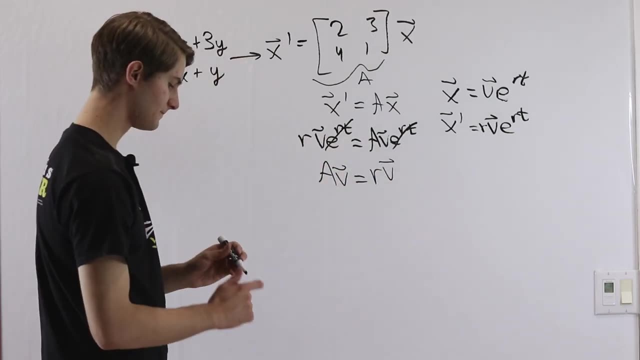 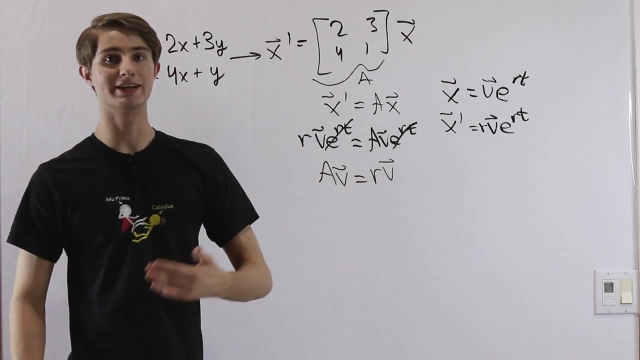 to nicely cancel out, And I'm just going to flip the sides of the equation here. that will leave us with a v. this here equals r times v, And this is another equation that we'll recognize, Because this is the exact equation for defining the eigenvalues of a matrix A. Again, you. 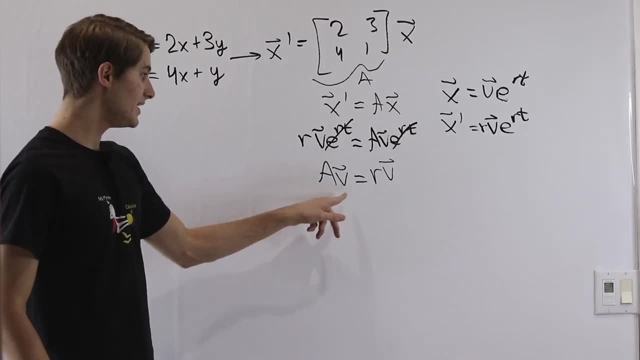 can check the video in the description for that. Normally we would write a v equals lambda v, but r is just a number like lambda. We're going to go through the same process. If we want to find the numbers r that satisfy this equation. all we have to do is find the 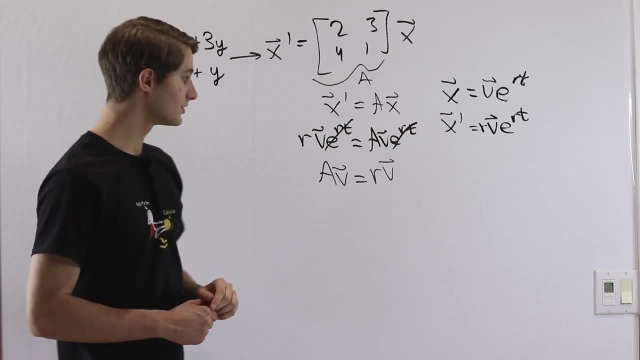 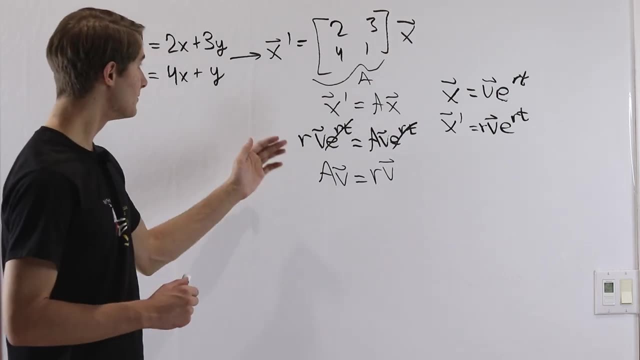 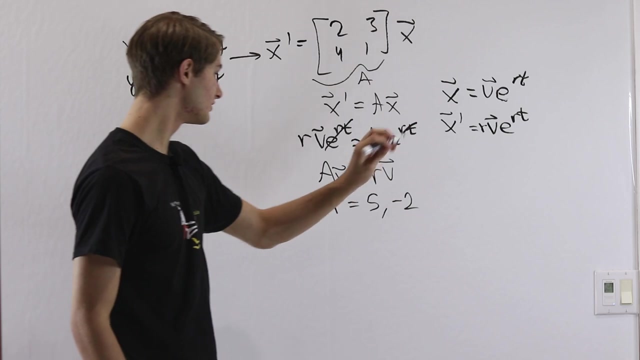 eigenvalues of our matrix A. So this is a differential equations class so I'm not going to go through how to find the eigenvalues. you can check the other video for that. But if we find the eigenvalues of this matrix they're going to be equal to five and negative two. And once we have the 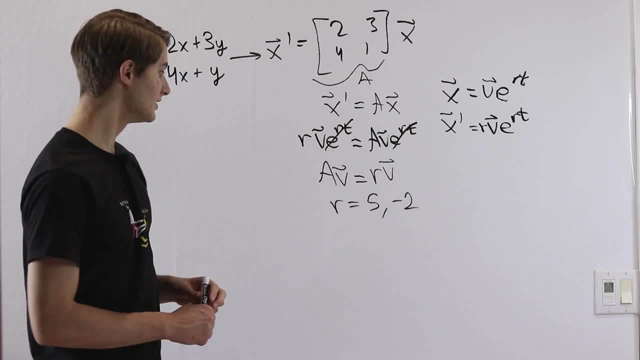 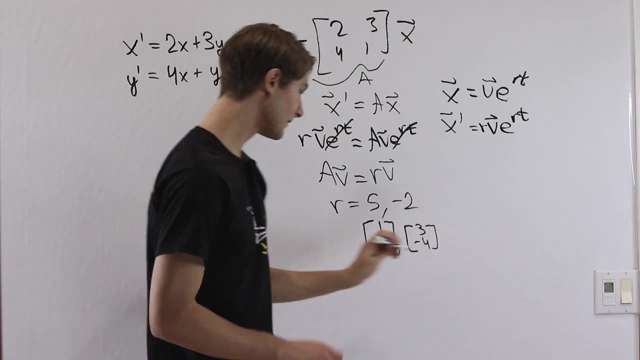 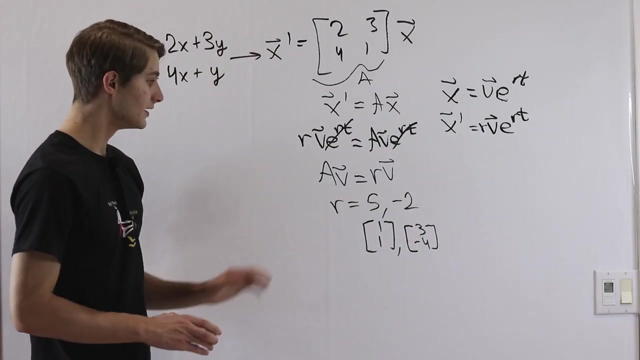 eigenvalues. then we go through and solve for the eigenvectors. The answers that we get for those are: one, one and three negative four. So one one goes with this eigenvalue, five, three negative four goes with this eigenvalue of negative two. This is actually. 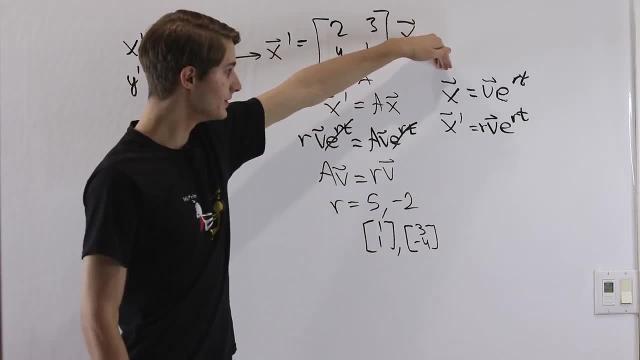 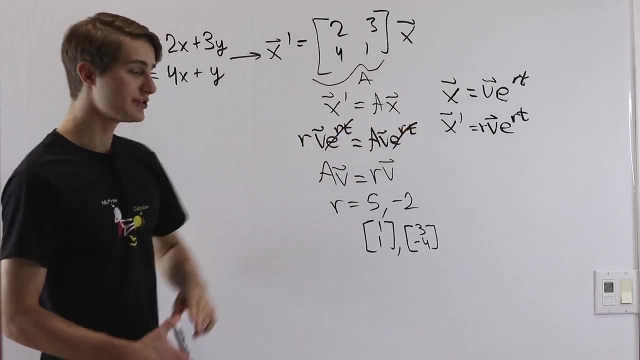 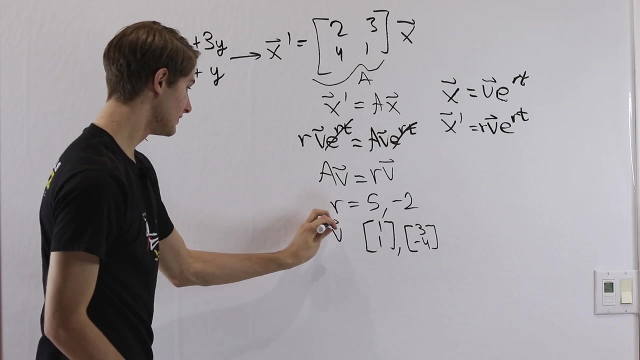 all the information that we need to solve for our original function x. So if we go back to our matrix equation here, x prime equals A x. the answer x that we're going to have is we're going to have the vector v, which is what we have here. These are the 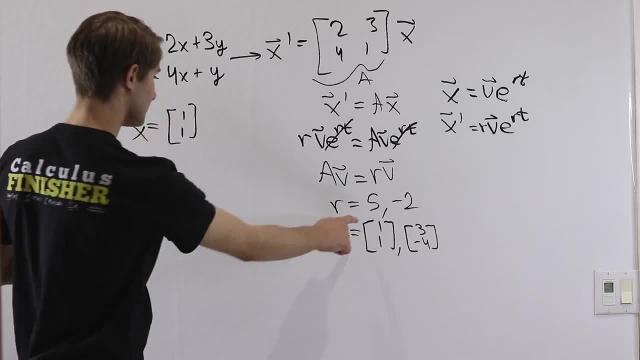 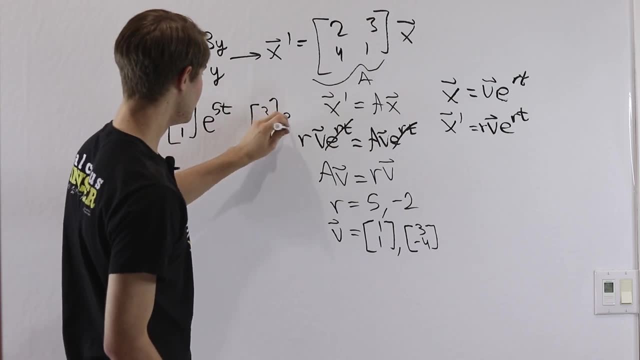 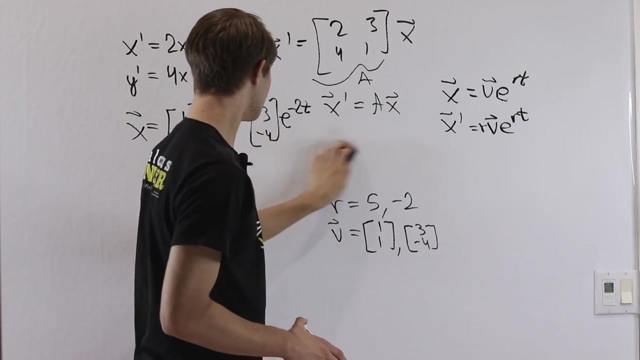 vectors v. So we have one one times e to the five t, And then the other solution we have is three negative four e to the negative two. So when we look at what we have here, notice that we have two different solutions, Remember. 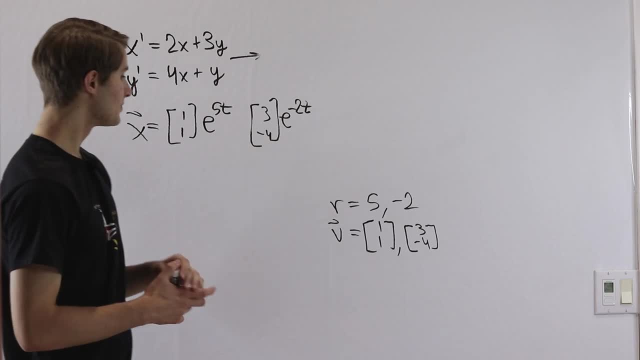 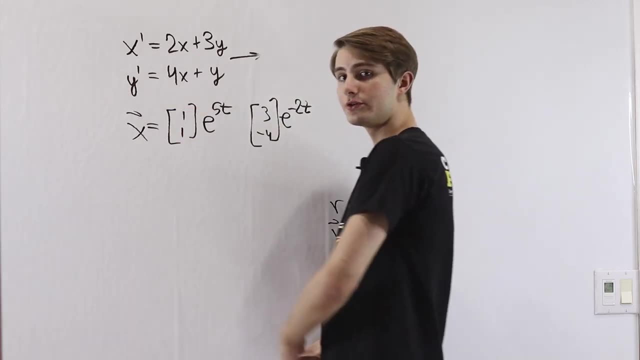 that each of these solutions is basically a complementary solution, Because if we look at this system of differential equations here and we move all the variables to the left side, they're all going to be equal to zero. So these are going to be homogeneous differential.